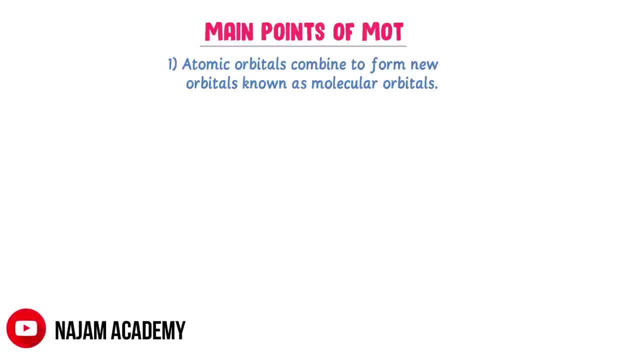 to form a new orbital known as molecular orbital. For example, consider these two hydrogen atoms. We know that this hydrogen atom has one as atomic orbital and this hydrogen atom has also one as atomic orbital. Now these two atoms of hydrogen would react chemically to form hydrogen molecule. Similarly, these 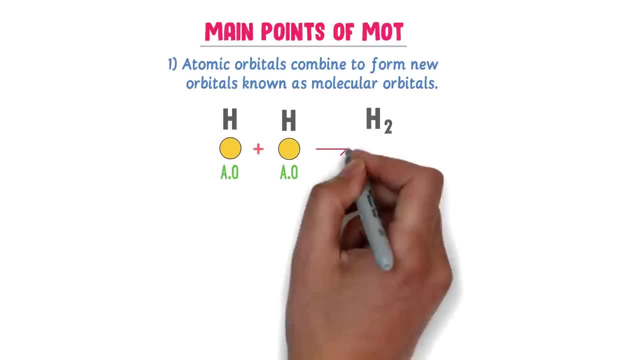 two atomic orbitals of hydrogen would overlap to form two molecular orbitals. Remember that when atomic orbitals, orbitals, overlap, they lose their identity and form molecular orbitals. Thus the first point of molecular orbital theory explains the formation of molecular orbitals from atomic orbitals. 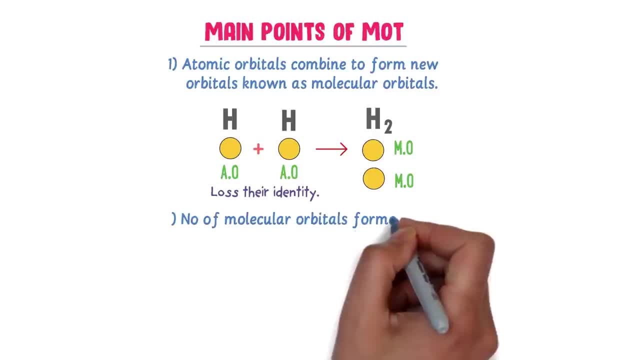 The second point of MOT states that the number of molecular orbitals formed are equal to the number of atomic orbitals combined are overlapped. For example, if two atomic orbitals overlap, it will form two molecular orbitals. If six atomic orbitals overlap, it will form six molecular orbitals. 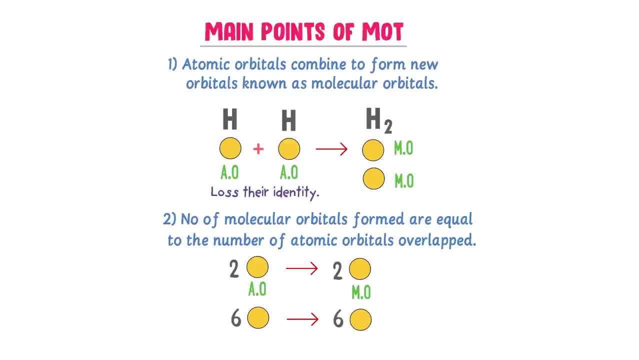 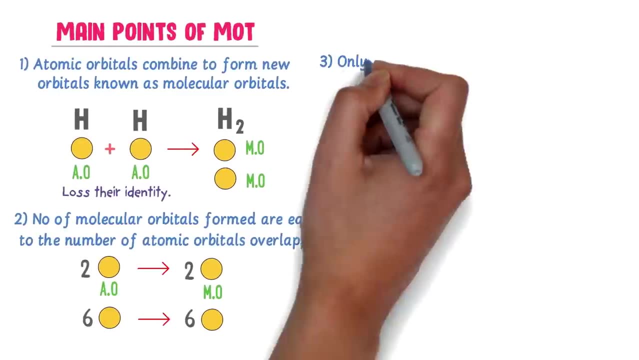 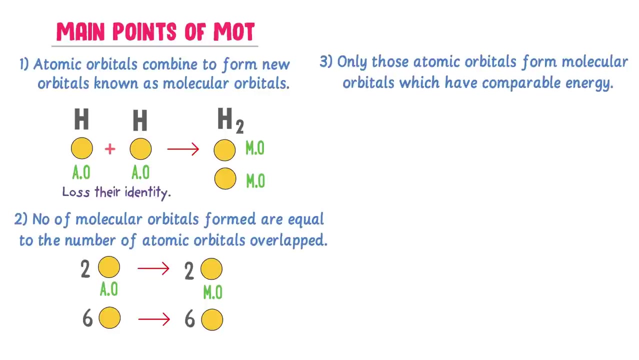 Thus, the second point of MOT is about the total number of molecular orbitals formed from atomic orbitals. The third point of MOT states that only those atomic orbitals combine together to form molecular orbitals which have comparable energy. For example, if the total number of molecular orbitals is equal to MOT, the total number 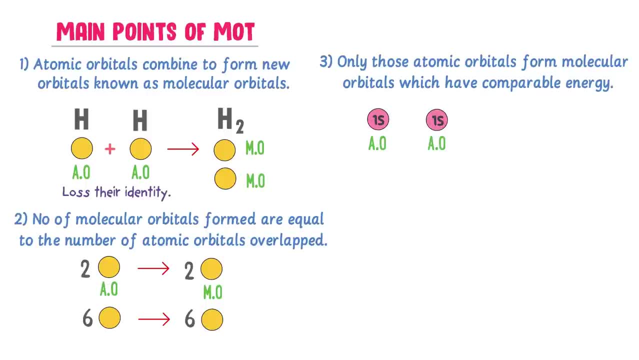 consider two 1s orbitals. These both atomic orbitals have the same energy, So these both atomic orbitals overlap to form two molecular orbitals of 1s. Remember that 1s atomic orbital and 2s atomic orbital do not combine or overlap to form a molecular orbital. It is because there 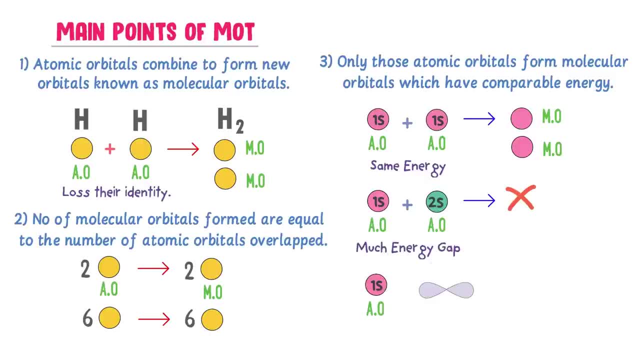 is much energy gap between them, Although 1s and 2p orbital can overlap to form molecular orbitals because there is less energy gap between them. Thus, the third point of MOT is about the energy gap and probability of overlapping of atomic orbitals. The fourth point of MOT states that 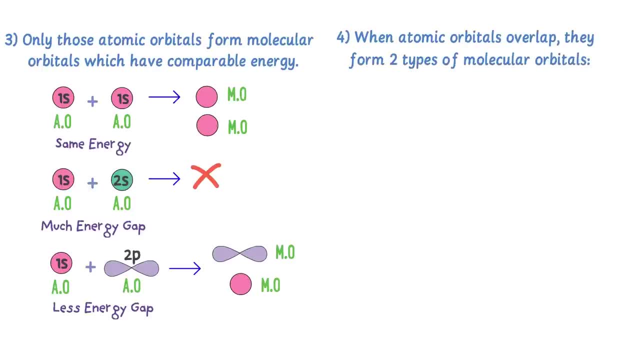 when two atomic orbitals overlap, they form two molecular orbitals. One is bonding molecular orbital And another is antibonding molecular orbital. For example, consider these two atomic orbitals: When they overlap, they form two molecular orbitals. This is bonding molecular orbital. 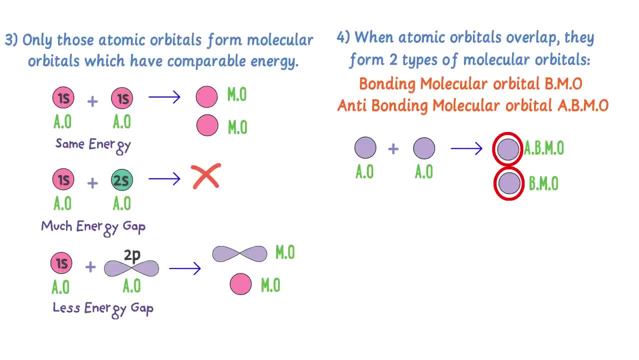 and this is antibonding molecular orbital. Thus, the fourth point of MOT is about the two types of molecular orbitals: bonding molecular orbital and antibonding molecular orbital. The fifth point of MOT states that bonding molecular orbital has lower energy than anti-bonding molecular orbital. 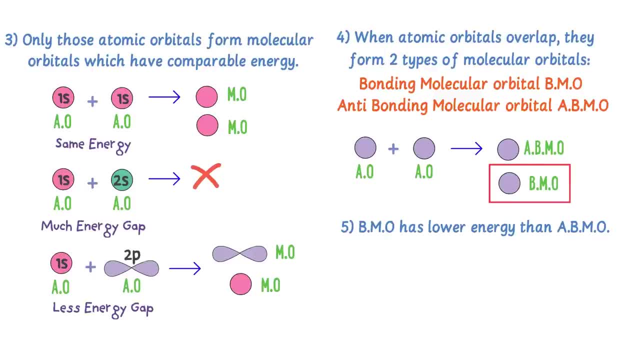 For example, the bonding molecular orbital is always placed below anti-bonding molecular orbital because bonding molecular orbital has lower energy and anti-bonding molecular orbital has higher energy. The sixth point of MOT states that axial overlapping of atomic orbitals form sigma, bond and parallel. 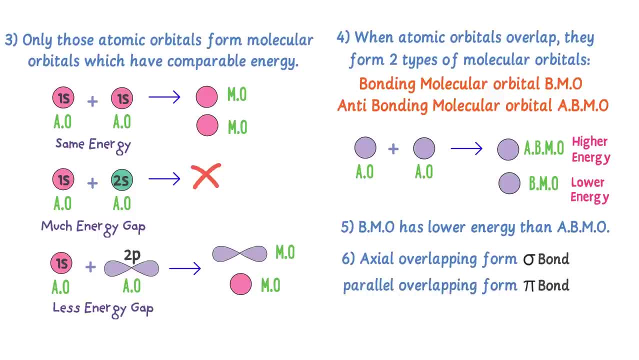 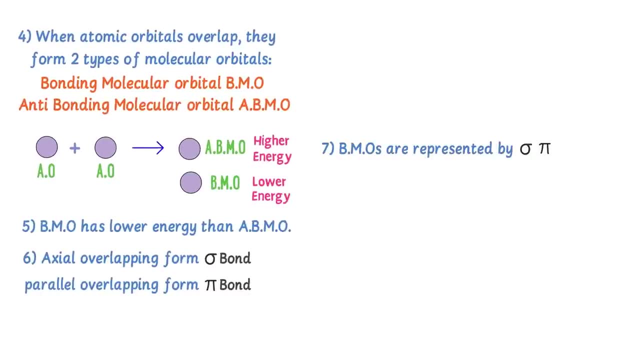 overlapping of atomic orbitals form pi bond. The seventh point of MOT states that the bonding molecular orbitals are represented by sigma and pi, while the anti-bonding molecular orbitals are represented by star sigma and star pi, For example. in this case, bonding molecular orbitals are represented by either sigma or 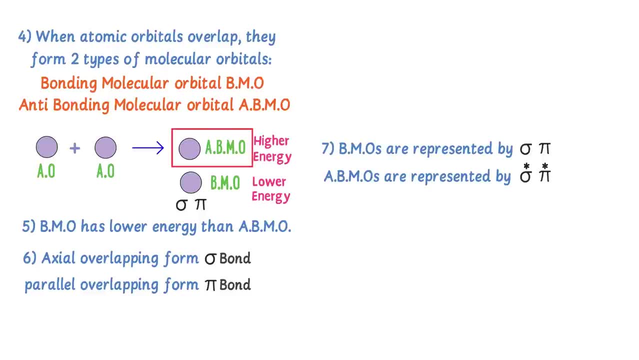 pi, while anti-bonding molecular orbitals are represented by either sigma or pi, Remember that the star on the sigma and pi shows the higher energy of anti-bonding molecular orbitals. Thus noted down, all these postulates are main points of molecular orbital theory. 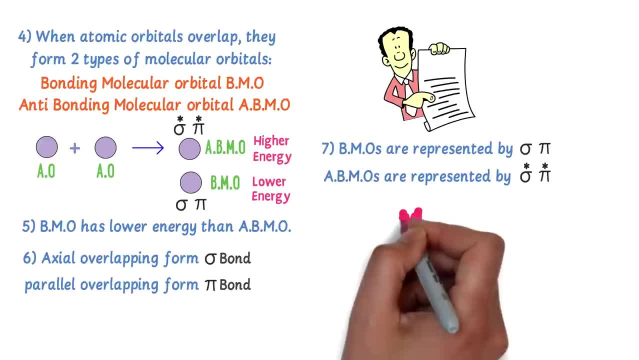 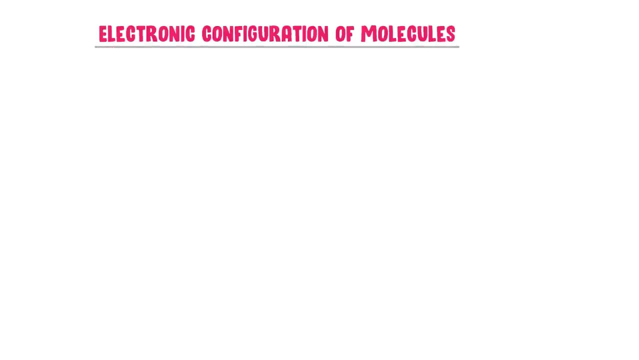 Now, as we learned in our previous slide, that molecular orbital theory explains the behavior of a molecule, I mean BBDSP. to learn the behavior of a molecule, we must understand the electronic configuration of a molecule. For example, consider two atoms of fluorine. 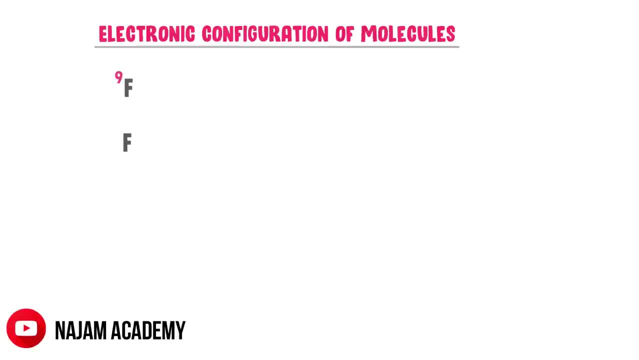 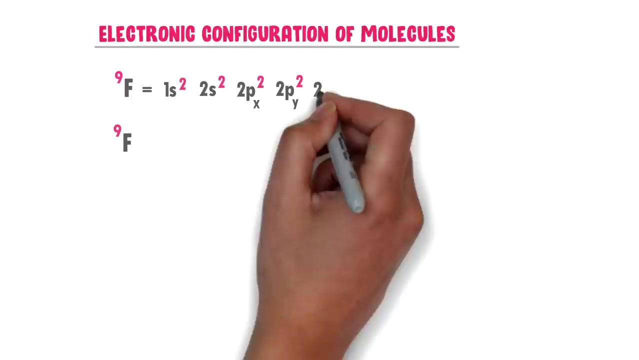 We know that the atomic number of fluorine is 9.. Now I do the electronic configuration of fluorine atom. 1s can accommodate two electrons, 2s can accommodate two electrons, 2px can accommodate two electrons, 2py can accommodate two electrons and 2pz can accommodate one electron. 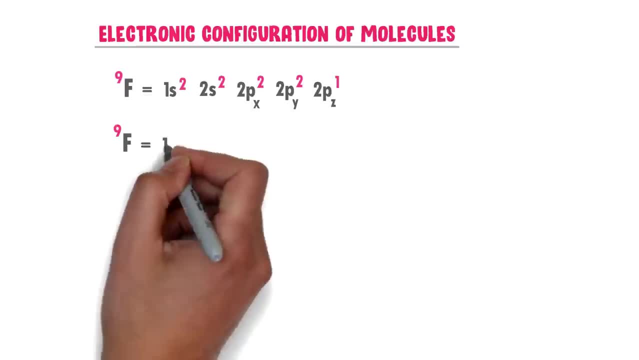 Similarly in the case of this fluorine atom. When fluorine contains the oxygen that has Monstrosian atoms. last image. Similarly in the case of this fluorine atom, Since fluorine contains full amount of oxygen, 1s can accommodate 2 electrons. 2s can accommodate 2 electrons. 2px can accommodate 2 electrons. 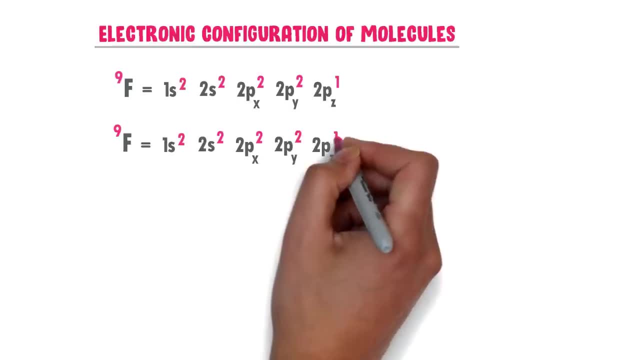 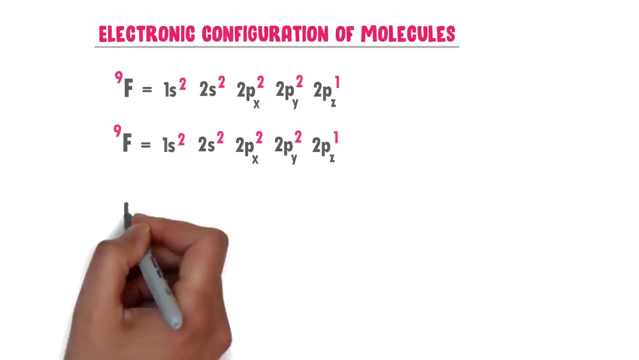 2py can accommodate 2 electrons and 2pz can accommodate 1 electron. We know that these two atoms of fluorine will react together chemically to form fluorine molecule, F2.. What about the molecular orbitals of fluorine molecule? 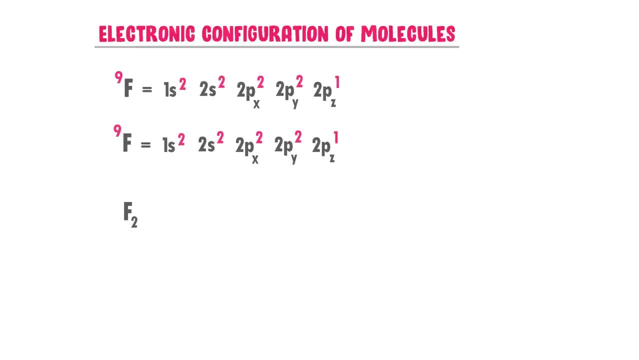 Well, we have already learned about them in molecular orbital theory. 1s atomic orbital of this fluorine atom and 1s atomic orbital of this fluorine atom would overlap to form two molecular orbitals, 1s and 1s. We already learned that one molecular orbital would be bonding molecular orbital and another. 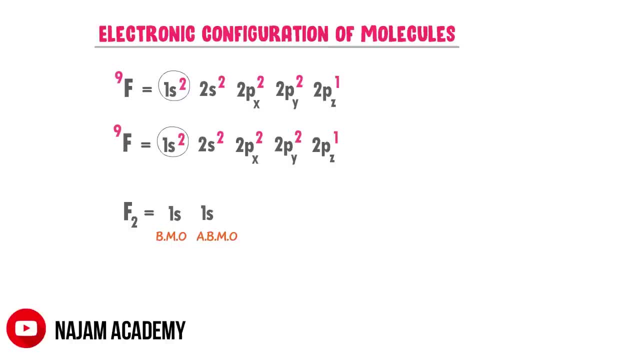 would be antibonding molecular orbital. Also, we put a star on Antibonding molecular orbital so two atomic orbitals of fluorine overlap to form two molecular orbitals. 2s. 2 electrons is accommodated in bonding molecular orbital. 1s and 2 electrons is accommodated. 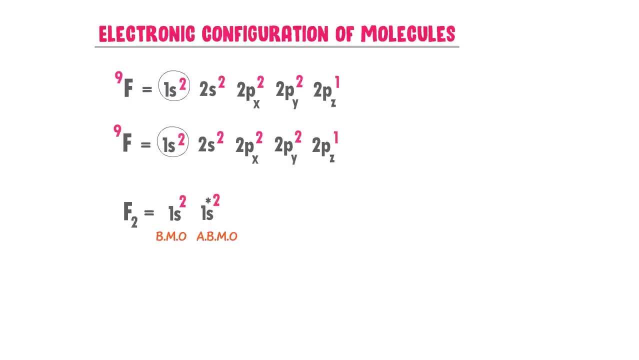 in anti-bonding molecular orbital, star 1s. Similarly, 2s atomic orbitals will overlap to form 2s molecular orbitals. 2 electrons is placed in this bonding molecular orbital and 2 electrons is placed in this anti-bonding. 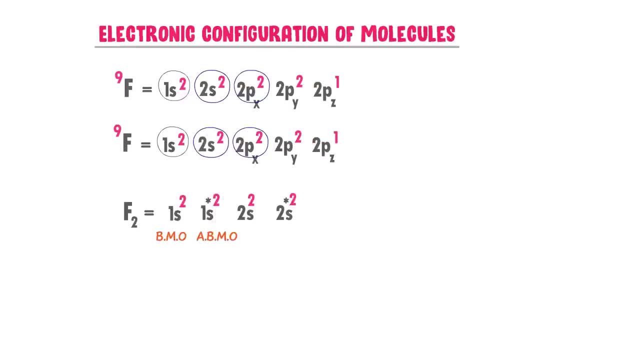 molecular orbital. 2Px atoms overlap to form two molecular orbitals. 2 Py atoms overlap to form two molecular orbital, and 2Pz atoms overlap to form 2pz molecular orbitals. Thus this is the electronic configuration of atom like fluorine, and this is the electronic. 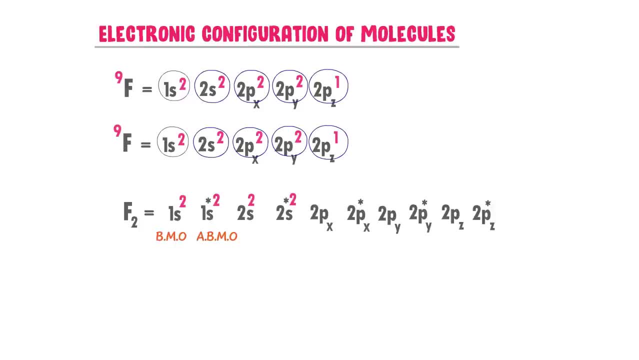 configuration of a molecule, like fluorine molecule. Remember that in case of electronic configuration of atom, We write time as 1s, 2s, 2px, etc. While in case of electronic configuration of a molecule, we write two times as 1s, 1s, 2s, 2s, 2px, 2px, etc. Therefore, noted down this important point, because a lot of students 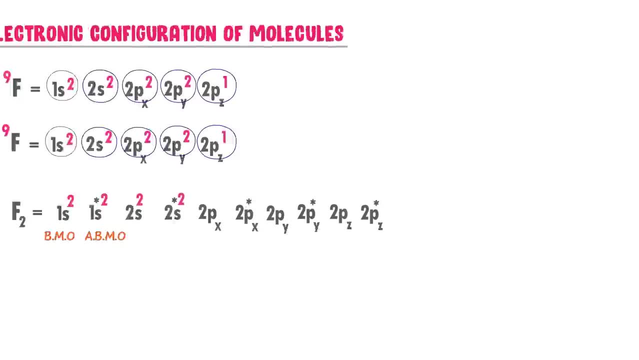 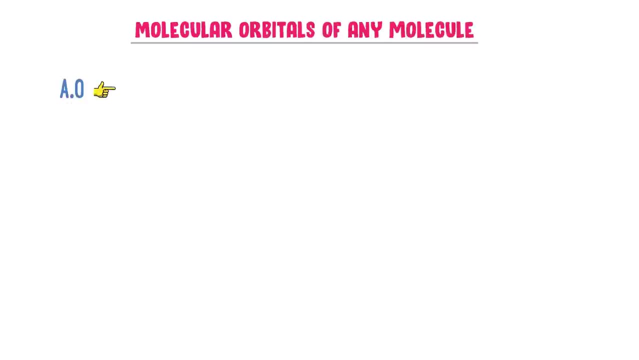 do not understand it. Now let me teach you my personal trick of writing molecular orbitals of any molecule. Firstly, I write atomic orbitals as 1s, 2s, 2px, 2py and 2pz. 1s atomic orbitals form. 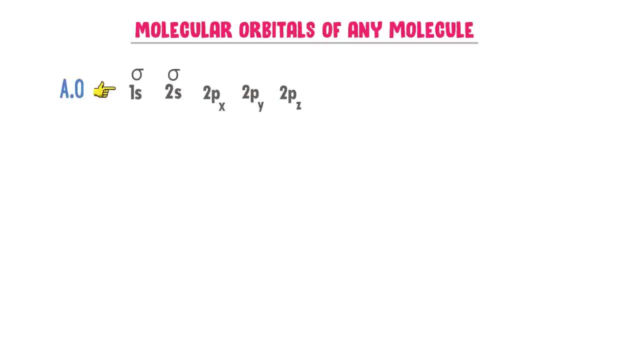 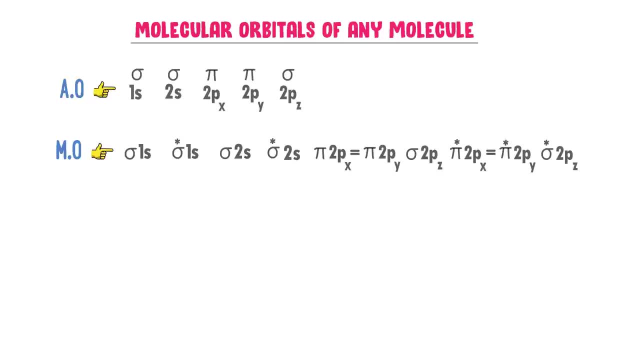 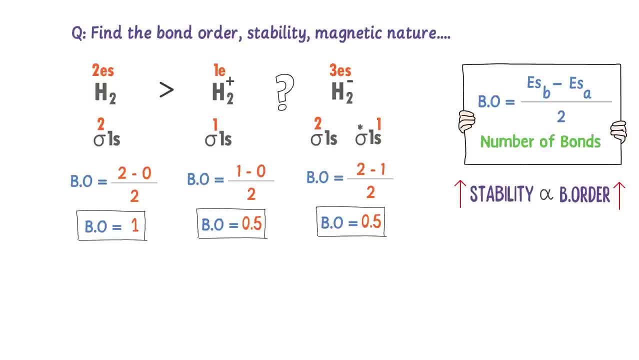 orbitals. Well, listen carefully. I write: 1s, 2px and 2py orbitals form sigma bond, Now positive ion and H2 negative ion, because they have the same bond order: 0.5, 0.5.. Well, if the bond order of two molecules are the same. we look at the number of electrons in antibonding molecular orbital. In case of H2 positive ion, there is no electron present in antibonding molecular orbital, While in case of H2 negative ion, there is one electron present in antibonding. molecular orbital. So H2 positive ion is more stable than H2 negative ion. Thus the order of stability is H2 molecule, H2 positive ion and H2 negative ion. Hence hydrogen molecule is more stable than H2 positive ion and H2 positive ion is more stable than H2 negative. 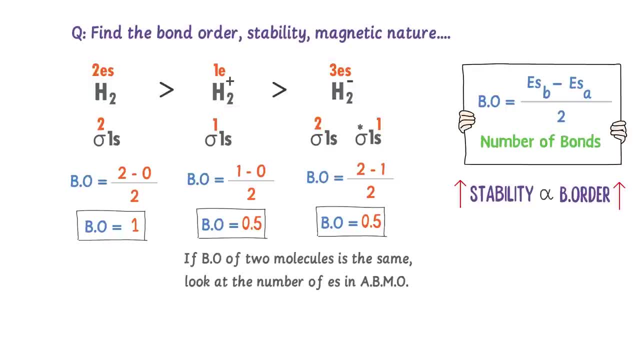 ion. Now, what about the magnetic nature of these molecules? Well, a molecule is paramagnetic if it has unpaired electrons, while a molecule is dimagnetic if it has paired electrons. Paramagnetic means that it is attracted by the magnet, while dimagnetic means that it 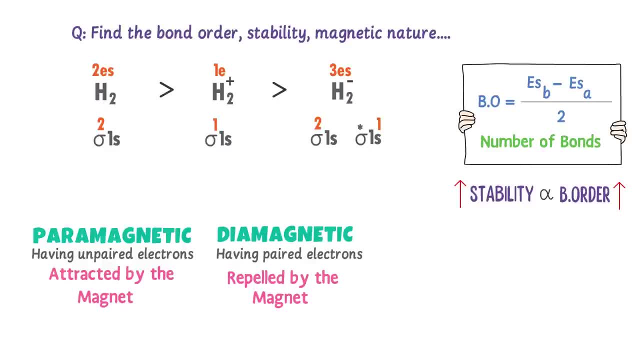 is repelled by the magnet. In case of H2 molecule, it has paired electrons, so it is dimagnetic. In case of H2 positive ion, it has unpaired electrons, so it is paramagnetic, While in case of H2 negative ion, it has also unpaired electrons, so it is paramagnetic. 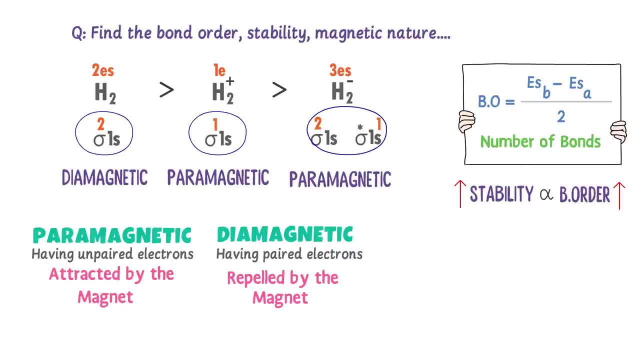 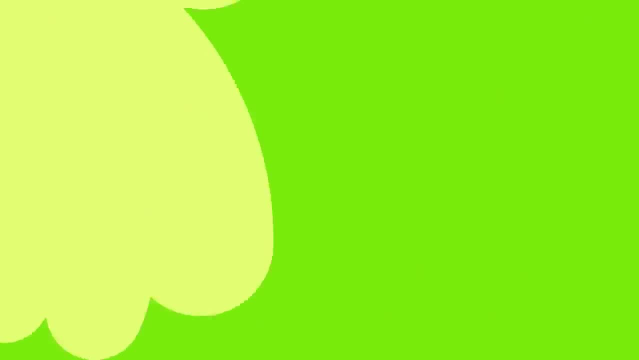 Thus molecular orbital theory successfully explains the bond order, stability and magnetic effect of all these molecules. Finally, let me draw the energy level diagram. When two 1s atomic orbitals overlap, they form one bonding molecular orbital sigma 1s and one. 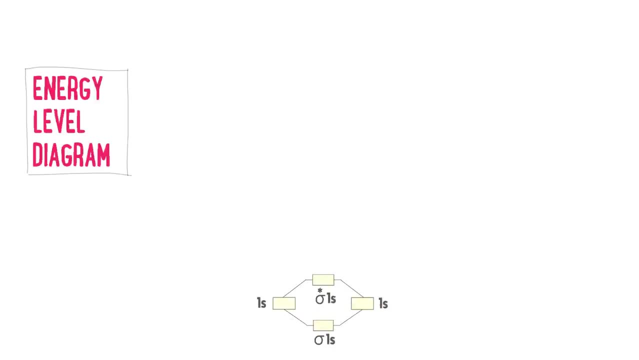 antibonding molecular orbital- sigma star 1s. When two 2s atomic orbitals overlap, they form one bonding molecular orbital- sigma 2s- and one antibonding molecular orbital- sigma star 2s. When two 2px, 2py, 2pz. atomic orbitals overlap, they form three bonding. 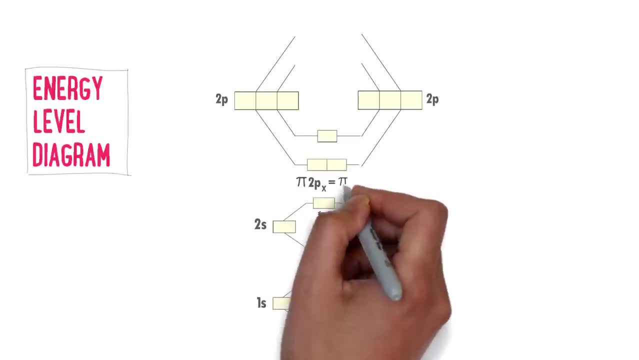 molecular orbitals pi 2px, pi 2py, because they have the same energy, one sigma 2pz molecular orbital, which has slightly higher energy than pi 2px and pi 2py, while they also form three antibonding molecular orbitals: pi star 2px, pi star 2py and sigma star 2pz. Also, 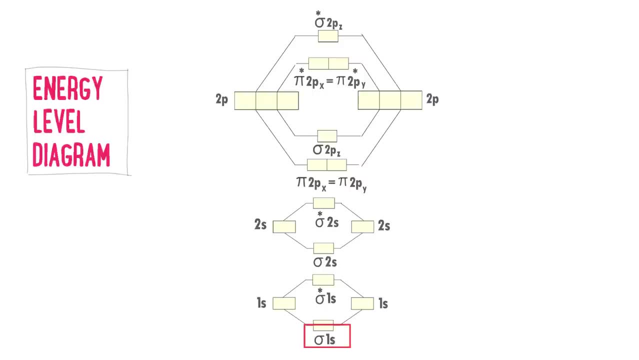 remember that sigma 1s bonding molecular orbital has low energy. 1s atomic orbital has more energy than sigma 1s, while sigma star 1s antibonding molecular orbital has higher energy than 1s atomic orbital, while sigma star 1s antibonding molecular orbital. 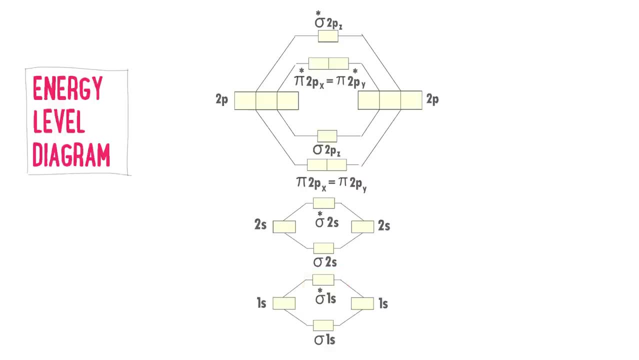 has higher energy than 1s atomic orbital. So the order of energy increases as you move up and sigma star 2pz has the highest energy. Thus, using this diagram, we can easily draw the energy level diagram of any molecule. For example, consider two nitrogen atoms. We know that the atomic number of nitrogen 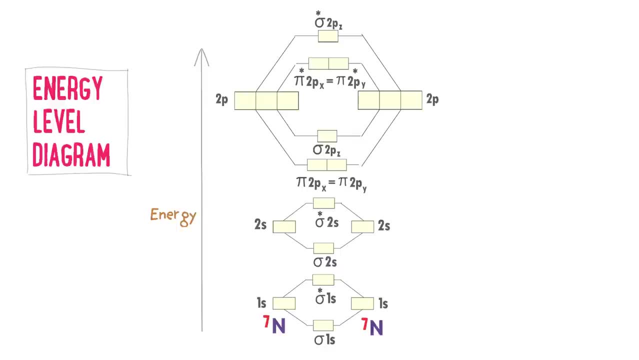 is 7.. So, in case of this nitrogen atom, two electrons are present in 1s, two electrons in 2s and the remaining three electrons are present each in 2px, 2py and 2pz. Remember. that these three electrons have the same energy level as sigma 2px, 2py and 2pz. So in case of this diagram we can easily draw the energy level diagram of any molecule. For example, consider the number of electrons present in sigma 1s. 2s atomic orbital has lower energy. than sigma 2px, 2py and 2pz. Or, in case of this diagram, we can easily draw the energy level, as sigma 2s atomic orbital has higher energy than 1s atomic orbital, while sigma star 2s antibonding molecular orbital has higher energy than sigma 2px, 2py and 2pz. 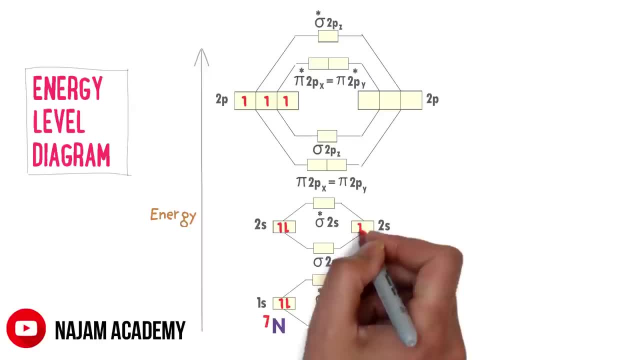 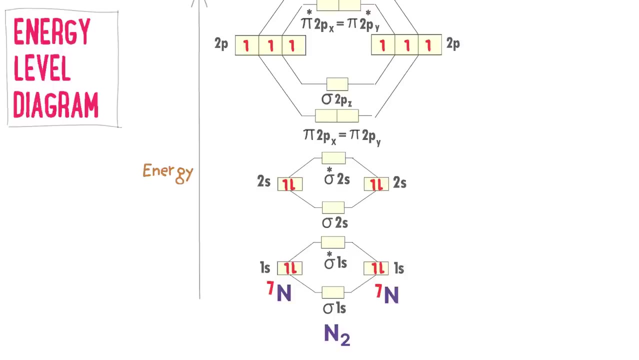 Similarly, in case of this nitrogen atom, two electrons are present in 1s, two electrons in 2s and the remaining three electrons are present each in 2px, 2py and 2pz, each having same spin. Now two atoms of nitrogen will react to form nitrogen molecule. We know.